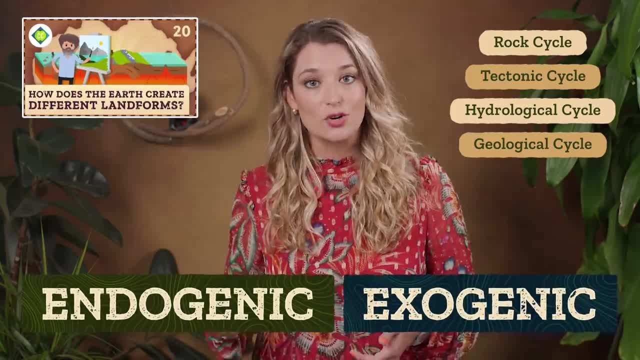 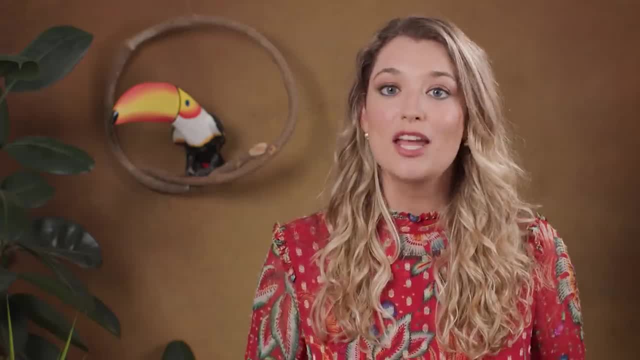 and take between the internal or endogenic system and external or exogenic system, which work in tandem to create, destroy and shape the Earth's crust. In particular, endogenic systems change the crust by increasing the relief or the local differences in elevation and are powered by heat at the Earth's core. 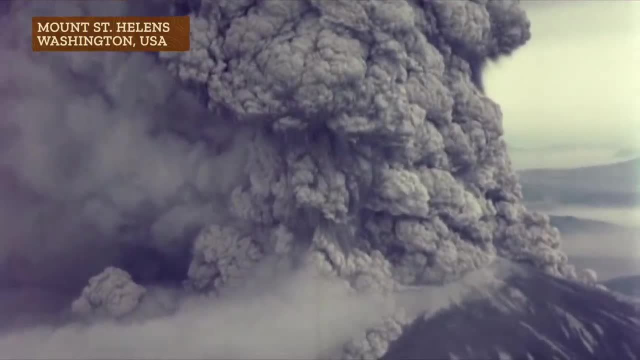 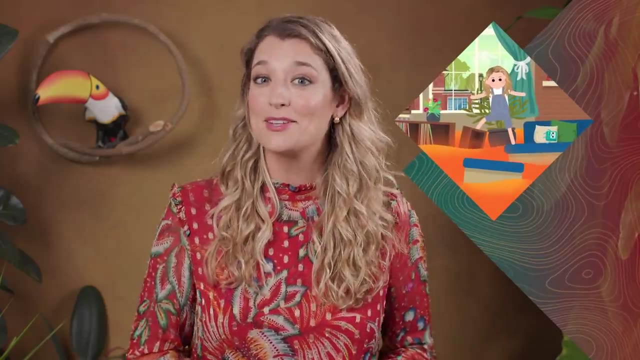 from decaying radioactive material, Which is where volcanoes come in. If you grew up in the US, like me, you probably played. The Floor is Lava, And if you haven't played it, I know what should be happening in your living room later today. 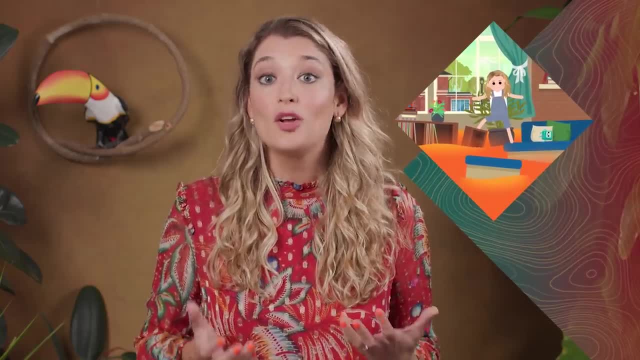 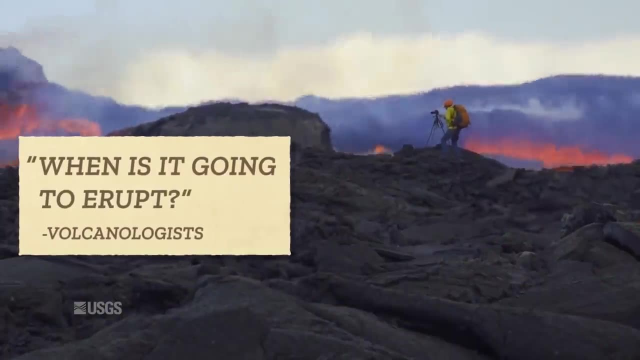 Lava holds some of the intense heat from the inside of the Earth, so it would be incredibly bad to have it threatening your home. So, looking at a volcano, one of the foremost questions in our minds is probably: when is it going to erupt, Especially for scientists who study volcanoes, or 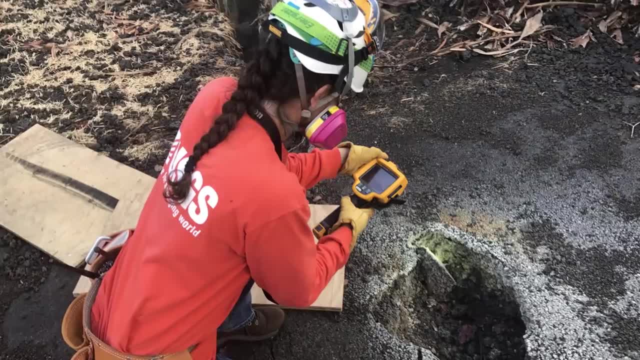 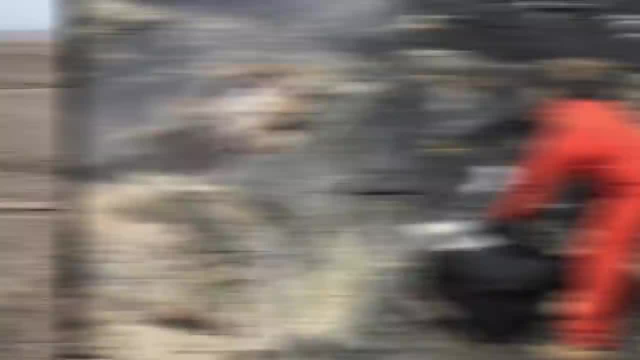 volcanologists. They look for clues both above and below ground that hint an eruption could happen, Like by examining millennia-old cooled rocks scattered about the volcano from past eruptions. These rocks show how the chemical makeup of the magma miles beneath the surface has changed and what might have happened before an eruption. 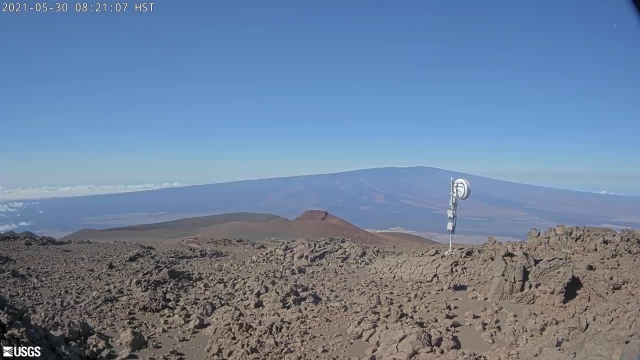 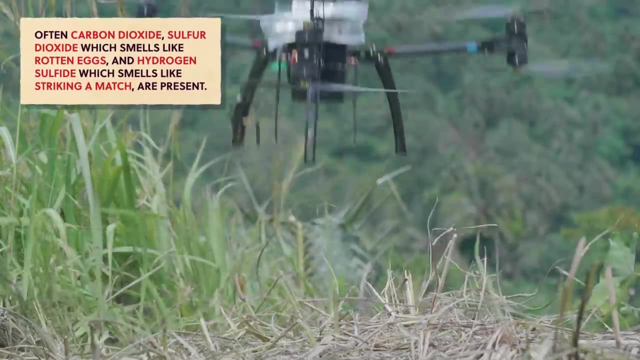 We can also look out for earthquakes, gravity and magnetic field changes or the ground starting to warp as magma or gases rise. As part of monitoring a volcano, we might go on a gas flight, which is a small airplane or drone flight, just to learn more about the gases being emitted as the volcano prepares to erupt. 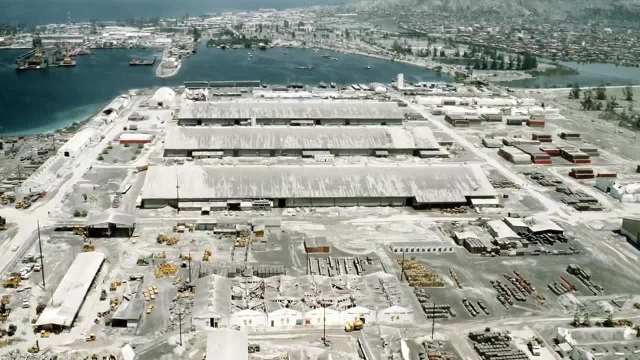 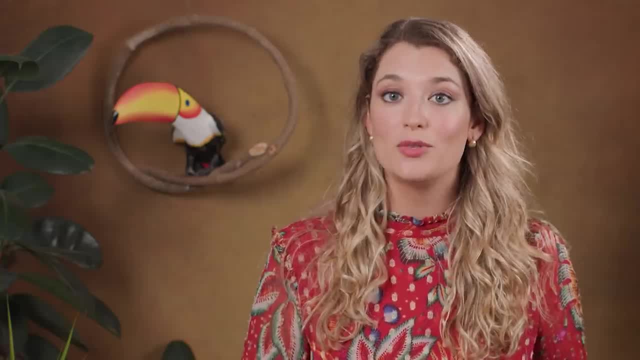 These techniques have helped us successfully predict eruptions and save thousands of lives, like when Pinatubo in the Philippines erupted in 1991.. But there's still more to learn. Research published in 2021 using satellite data showed that in the years leading up to an 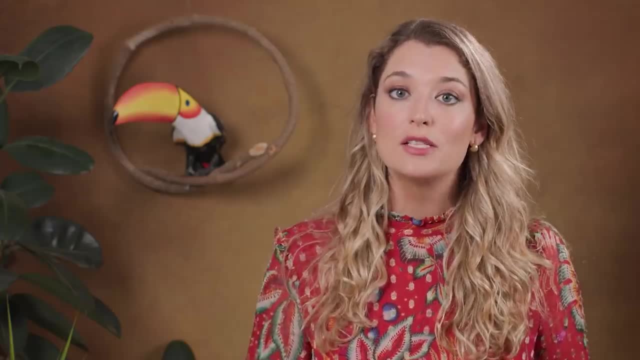 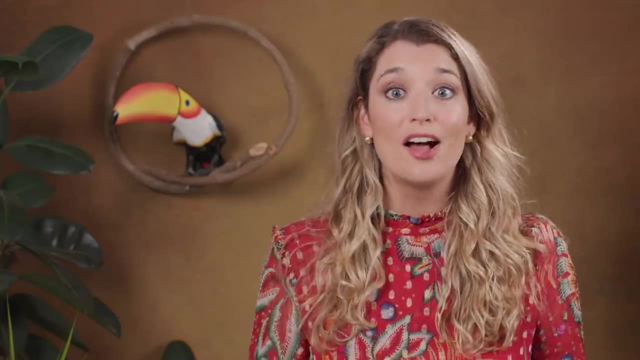 eruption, the temperature of the ground around the volcano can increase by up to about 1 degree Celsius. So monitoring ground temperature using satellite data could become a new predictive tool and help get more people out of harm's way. But while predicting volcanic activity is still difficult, we at least know where volcanoes 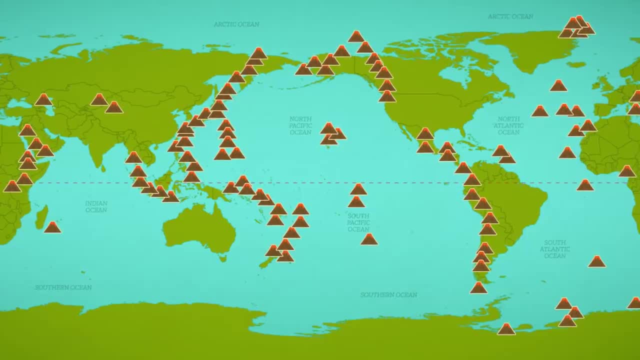 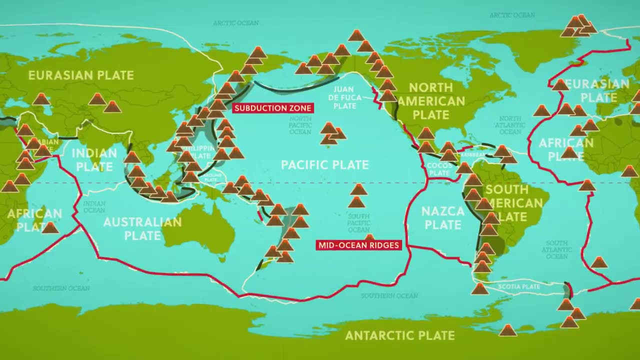 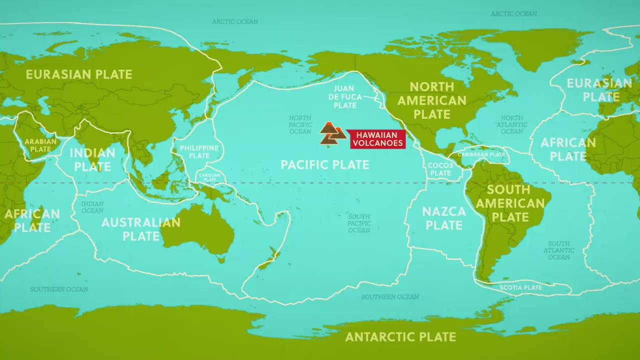 are? Their locations follow a definite pattern. Mostly, Most volcanoes are located above subduction zones, where two plates are converging and one dives under the other, and at mid-ocean ridges, where the seafloor is spreading. But a few occur within plates, Like the Hawaiian volcanoes, which sit in the middle of the Pacific. 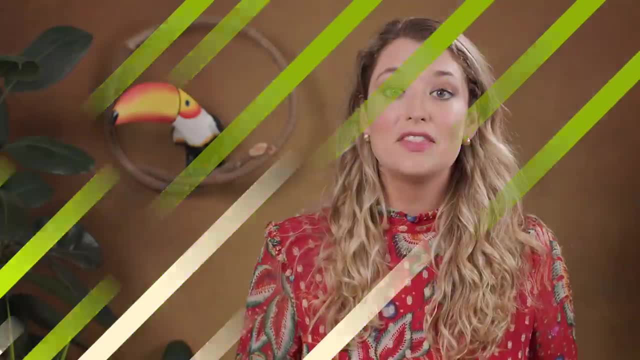 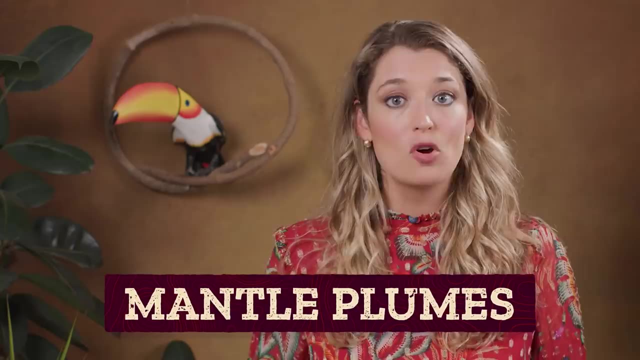 Plate, thousands of kilometers from the closest plate boundary. Some of these mysterious volcanoes seem to be driven by mantle plumes, which are special features that can be hundreds of kilometers across, where abnormally hot magma can rise up through the mantle and melt crustal rock into more magma. 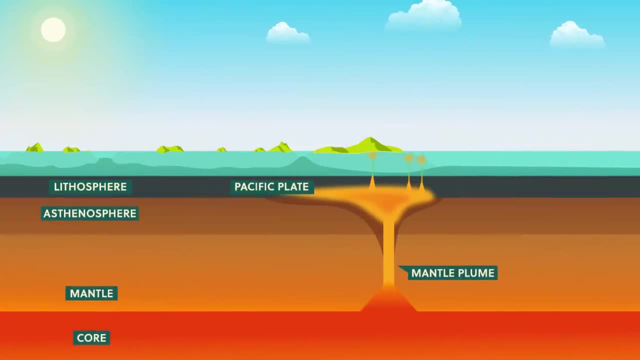 We're still figuring out how mantle plumes work, but one common school of thought is that they get their start at the core-mantle boundary. The outer core provides the extra heat that helps the magma get pumped up into the mantle. It's like a glob of hot material that sits at the end of a stalk of. 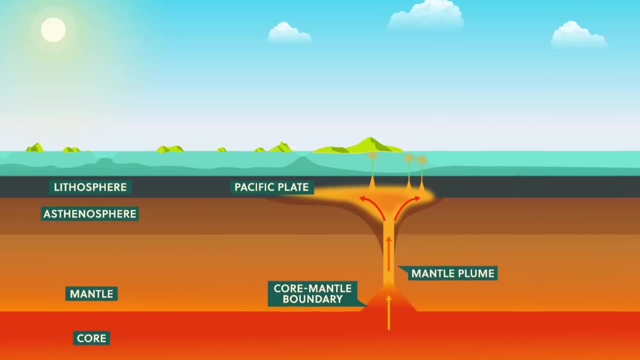 inside-Earth stuff with its base in a giant magma chamber, which is like a liquid vat of magma deep within the Earth, And it literally melts a path as it moves upwards to the lithosphere, Near the lithosphere, the top of the plume. 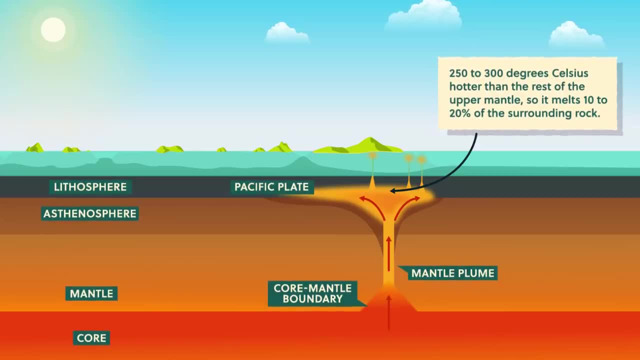 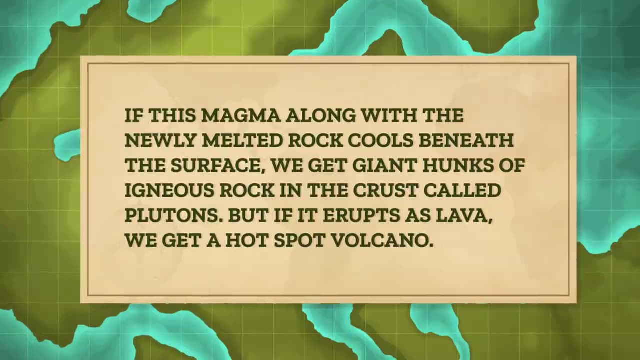 mushrooms and spreads out. Here the plume temperatures can be 250 to 300 degrees Celsius hotter than the rest of the upper mantle, so it melts 10 to 20% of the surrounding rock. If this magma, along with the newly melted rock, cools beneath the surface, 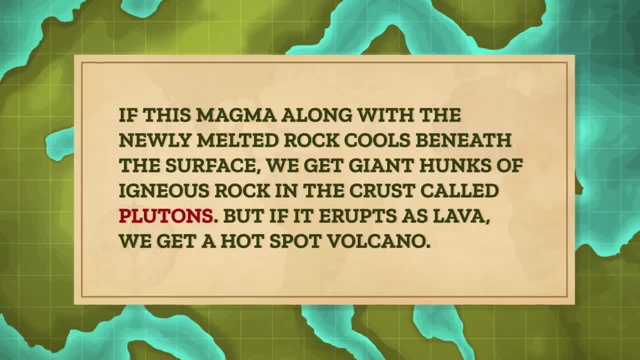 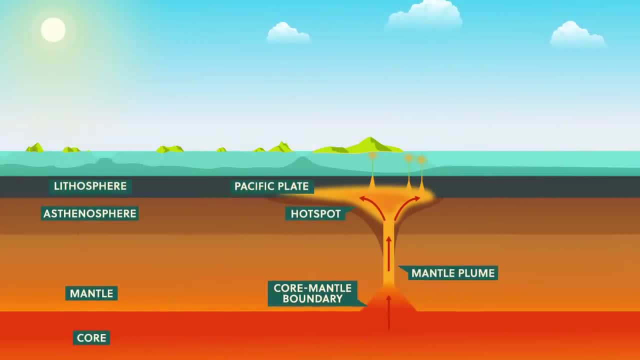 we get giant hunks of igneous rock in the crust, called plutons, But if it erupts as lava, we get a hotspot volcano Or even a trail of hotspot volcanoes. Most of the time, a mantle plume stays fixed while a plate slides slowly over it. which spreads out the volcanic activity, Like beneath Yellowstone National Park in the middle of North America, there's a hotspot that's created a 500-mile trail of more than 100 calderas, which are giant craters left after a volcano has collapsed, often after exploding. 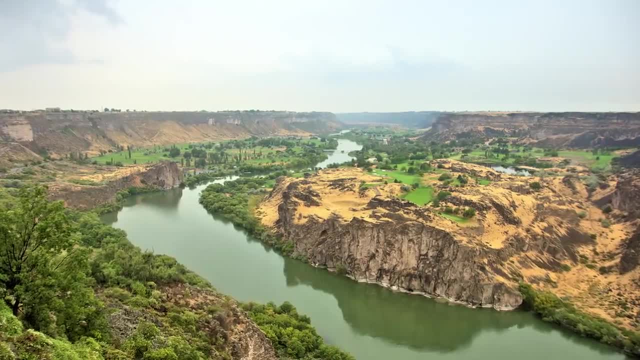 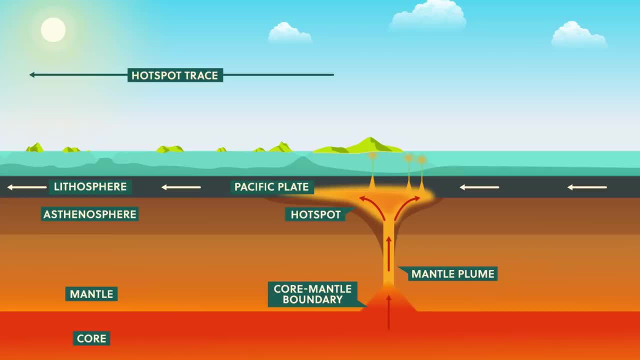 They once generated enormous volumes of basaltic lava across Idaho's Snake River Plain. In the ocean, plates moving over hotspots can produce a chain of volcanic islands or a hotspot trace, Like the Hawaiian Islands formed as the Pacific Plate moved across a hotspot for almost 80 million years, producing a string of 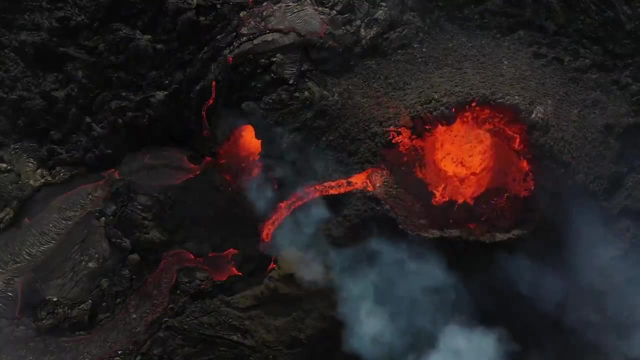 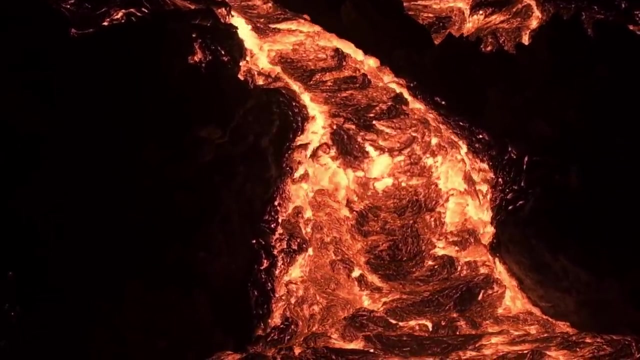 volcanic islands, each older than the one after it, But whether located above hotspots or on plate boundaries, volcanoes are kind of like windows into the center of the Earth, which helps us understand more about how it all works. Throughout our planet's history, volcanism even helped to produce the atmosphere by emitting. 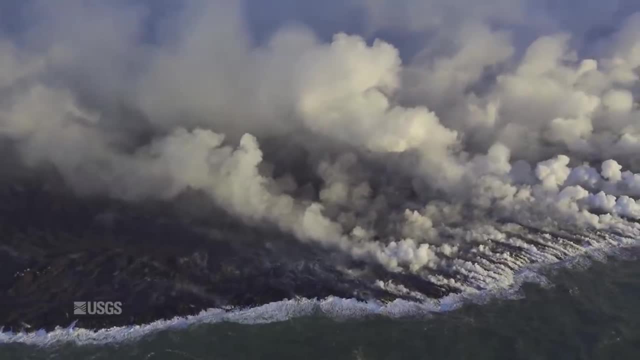 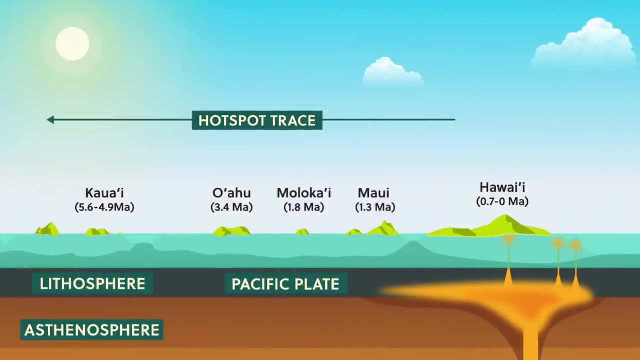 gasses stored in the Earth's interior And the molten materials spewed by volcanoes creates new igneous rocks which make up approximately 90% of the Earth's crust. Like, the oldest of the 8 main Hawaiian islands is Kauai, which is about 5 million years old, And Hawaii itself is the oldest of 8 main Hawaiian islands And Hawaii itself, like Kauai, is the oldest of 8 main Hawaiian islands is Kauai, which is about 5 million years old, and Hawaii itself, which is about 5 million years old, and Hawaii itself. 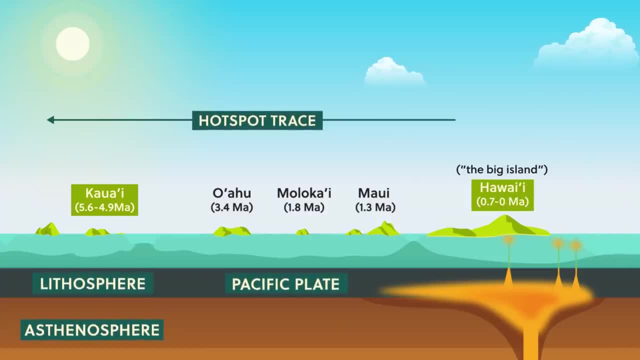 itself, which is sometimes called the Big Island, took less than half a million years to build, But the baby in the hot spot trace is an underwater mountain called a seamount. that's still about 975 meters from the ocean surface. Its name is Lohi, but it won't see the sun for another 10,000 years or more. 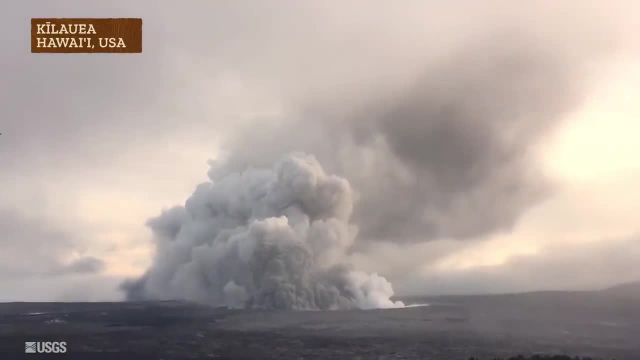 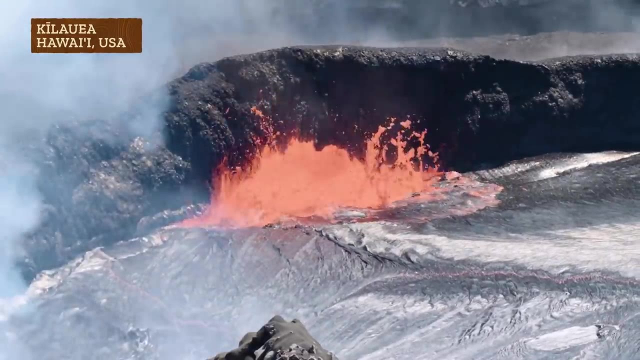 So, geologically speaking, Hawaii is still growing. The volcano called Kilauea in Hawaii has been nearly continuously erupting since 1983. But it doesn't make a lot of headlines because the eruptions here don't typically come with a lot of volcanic activity fireworks. 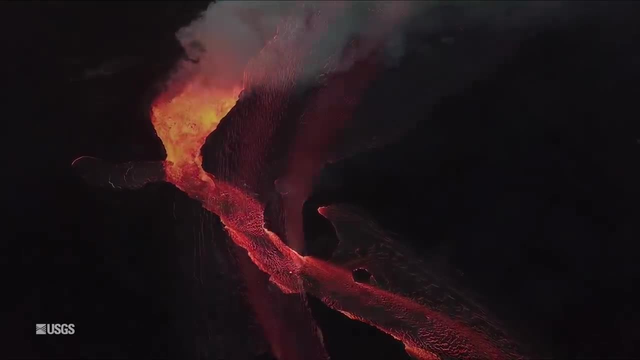 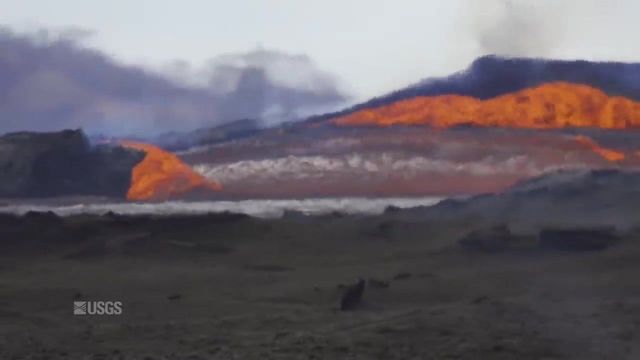 Which is actually telling us something about the volcano and the crust being formed. The magma from Kilauea has a specific chemical makeup which determines how fluid it is or its viscosity. Magmas which built the Hawaiian islands are mafic lavas. 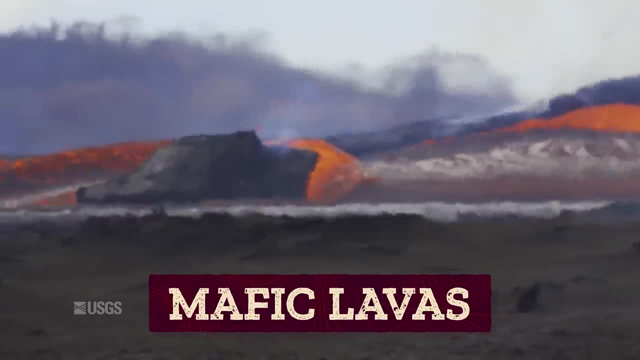 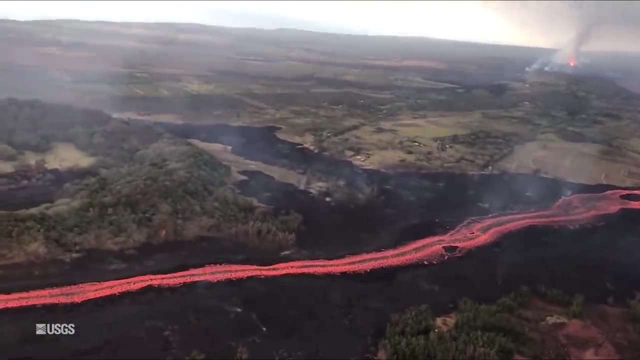 They have a low viscosity and are very fluid or runny and don't hold a lot of gas. Without the extra gases, the pressure doesn't build up as much and we get a quiet eruption. This allows the lava to travel long distances and spread out in thin layers. so Kilauea is. 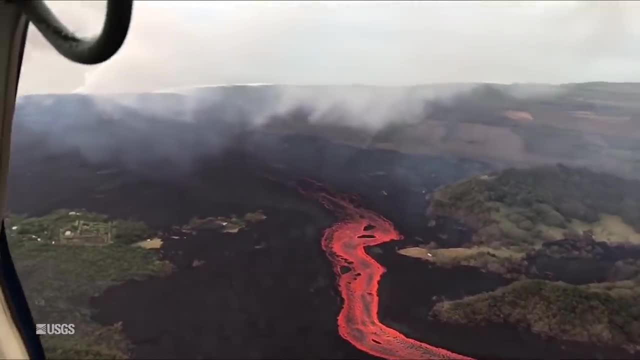 aptly known as the Kilauea volcano. Kilauea is often named because it's often thought to mean spewing or much spreading. The mafic and basaltic lavas cool to form a dark basaltic rock which is low in silica. 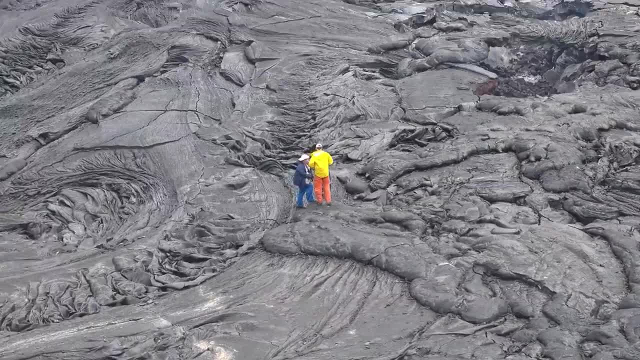 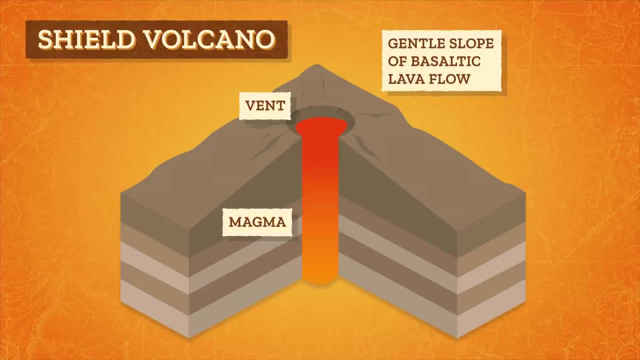 and rich in iron and magnesium. These minerals make the crust heavier and denser, and basaltic lava helps make up the bulk of the ocean floor. The magma shapes the volcano too. We get a broad, rounded dome with gentle slopes that looks like a warrior's shield, which 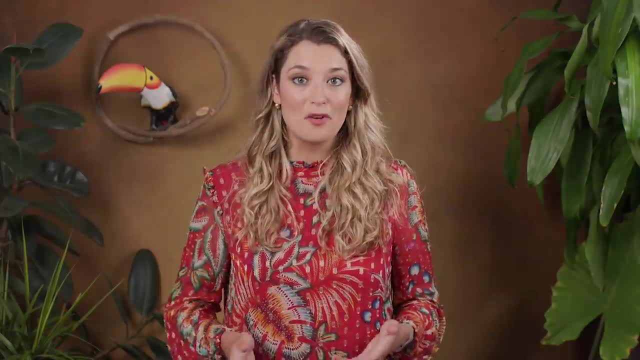 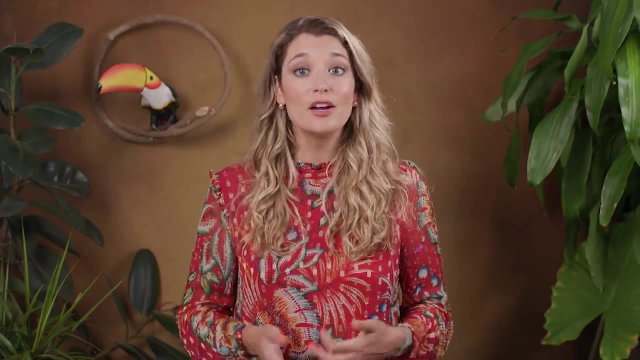 is why they're called shield volcanoes. So the Hawaiian volcanoes are hotspot volcanoes because of where they're located, But they're also the most famous of shield volcanoes because they're known for their type of eruption. In fact, Mauna Loa on the island of Hawaii is the world's largest active volcano. 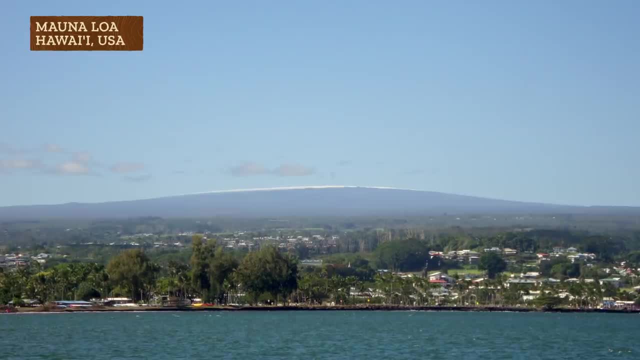 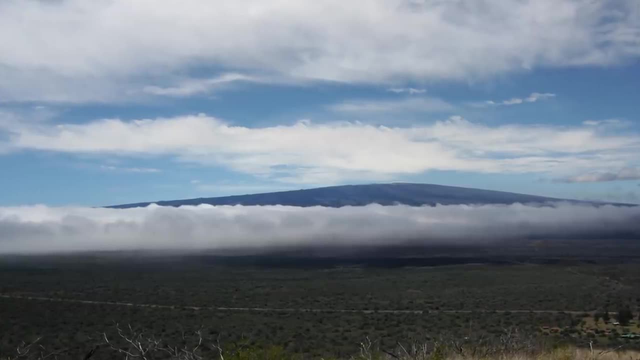 In Olelo, Hawaii. Mauna Loa means long mountain, which makes sense when we look at its profile, with its smooth slopes rising to a broad-topped volcano. Hawaiian volcanoes can rise 4,000 meters above sea level, but are actually more than twice. 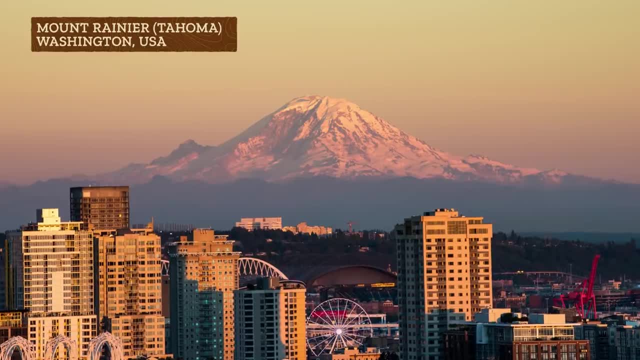 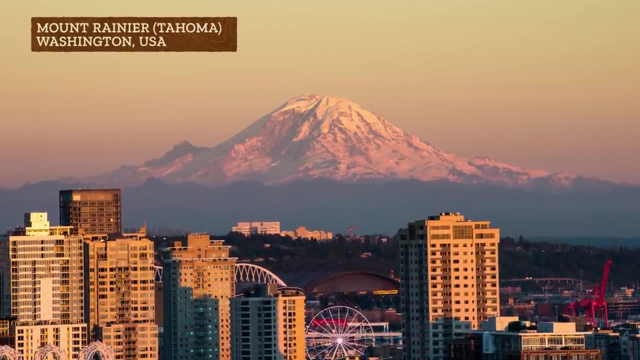 that high. if we include the portion below sea level And if we compare this gentle giant to the height of explosive Mount Rainier, which is southeast of Seattle Washington in the Cascade range of volcanoes in the US, the difference is striking and hints at the fact that they actually have different tectonic. 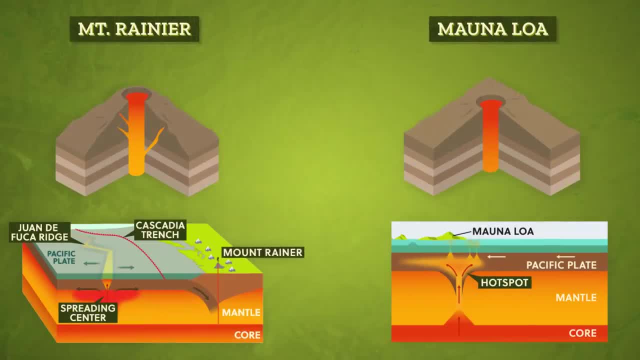 origins. Unlike Mauna Loa over a hotspot, Mount Rainier was created when the lighter continental crust of the North American Plate collided with and subducted the denser oceanic crust of the Juan de Fuca Plate, Because hundreds of meters of sediments are often carried along when a plate is subducted. 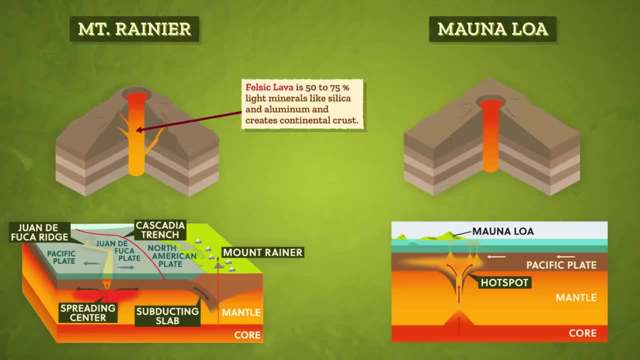 and melted into magma, it produces a felsic lava which is 50 to 75% light minerals like silica and aluminum and creates continental crust. So the magma from Mount Rainier is thicker than magma from the North American Plate, which is 50 to 75% light minerals like silica and aluminum and creates continental crust. 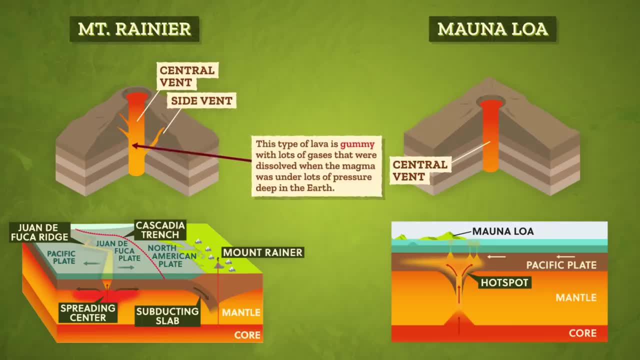 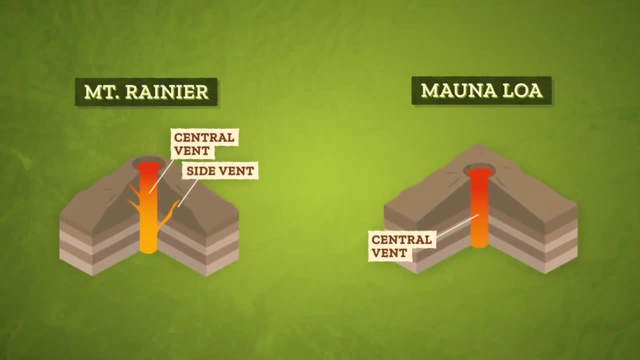 So the magma from Mount Rainier is thicker than magma from volcanoes like Mauna Loa. This type of lava is gummy with lots of gases that were dissolved when the magma was under lots of pressure deep in the Earth. When too much gas accumulates within the magma chamber, the pressure grows and grows. 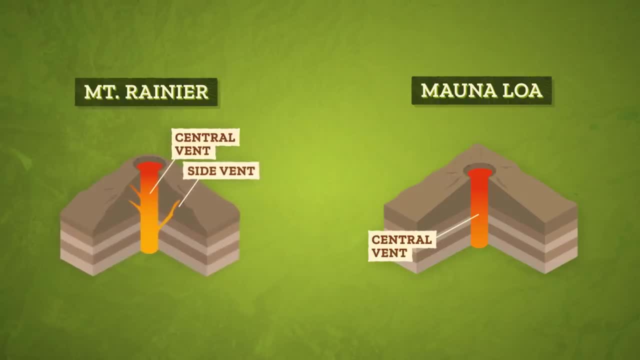 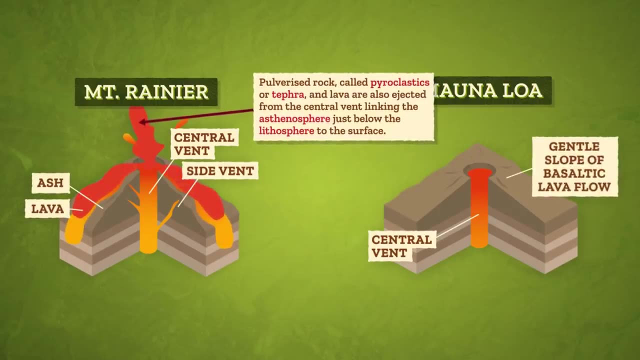 Then, as molten rock rises to the surface, the pressure is lower, so the gases expand in a violent blast. Pulverized rock, called pyroclastics or tephra, and lava are also ejected from the central vent linking the asthenosphere, just below the lithosphere, to the surface. 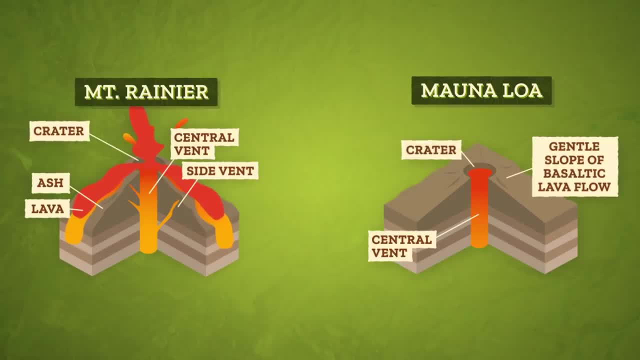 It all starts to fall outside the crater, Or a bowl-shaped depression that usually forms at the summit around the base of the volcano. Alternate layers of tephra and lava, which doesn't flow very far from the volcano, produce a composite or stratovolcano with a tall cone shape that steepens towards the. 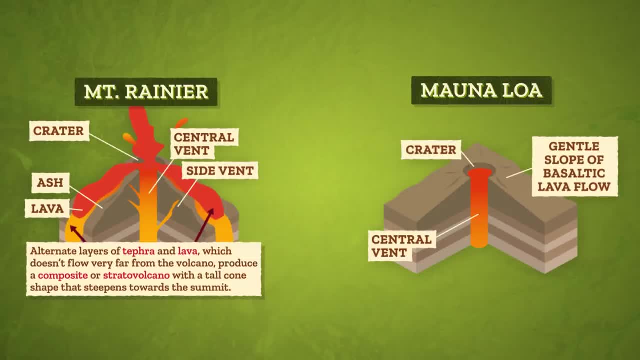 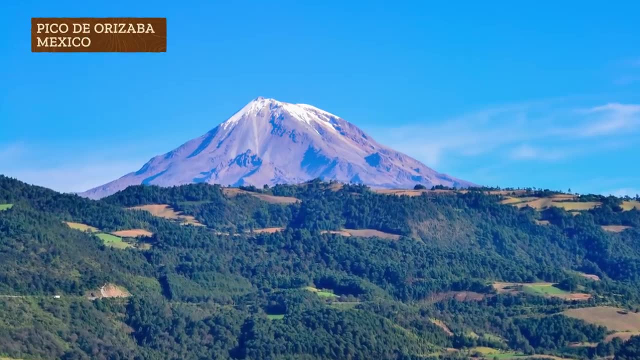 summit. So we get the classic symmetrical volcano of our imaginations, like Mount Mayan in the Philippines, Mount Fuji in Japan, Mount Shishaldon in Alaska and Pico de Orizaba in Mexico. We've been mainly talking about terrestrial volcanoes or volcanic activity on land, but 70% of volcanic activity on land is actually volcanic activity on land. So we get the classic symmetrical volcano of our imaginations, like Mount Mayan in the Philippines, Mount Shishaldon in Alaska, Mount Shishaldon in Alaska and Pico de Orizaba. 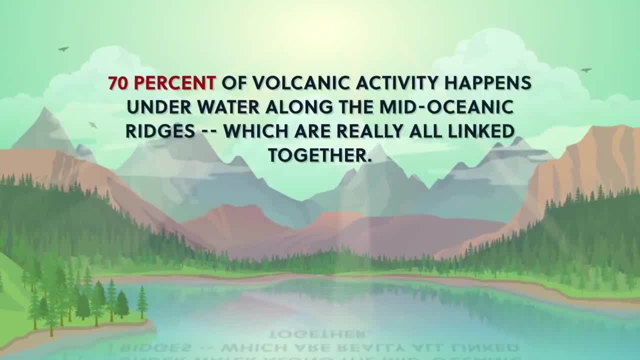 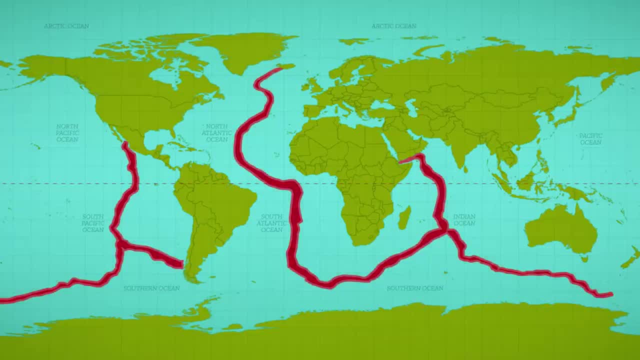 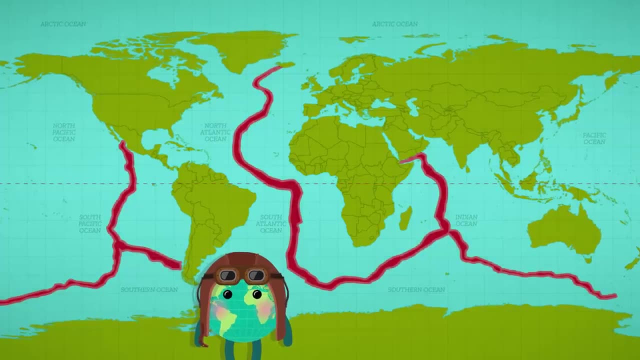 in Mexico, And we can think of the mid-oceanic ridge, all 60,000 kilometers of it, as one vast volcano stitched together like the seams of a baseball snaking along the ocean floor. Some physical geographers even call it the most important feature on the Earth's surface. 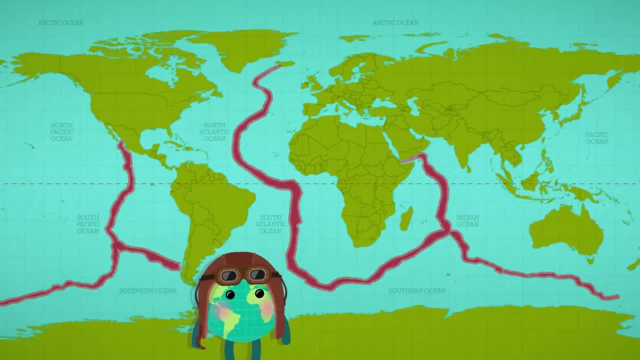 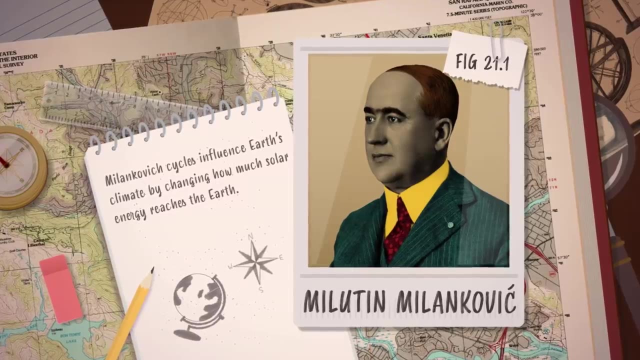 And acoustic data from 9 seabed eruptions along this ridge has opened up a whole new perspective on how the Earth works. We know that Milankovitch cycles explain how the Earth has switched between glacial and interglacial periods throughout the most recent ice age in Earth's geological history. 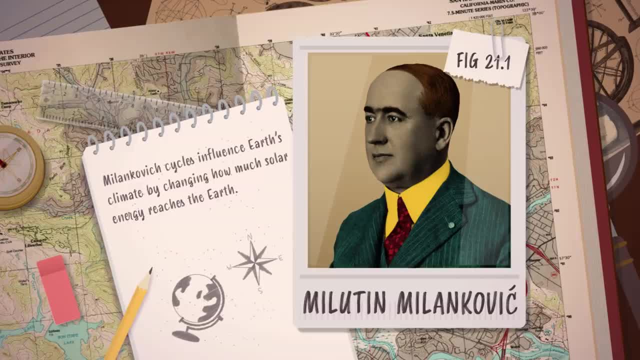 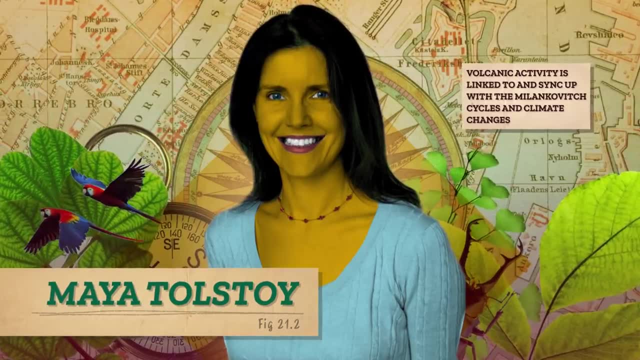 Changes in the wobble and tilt of the Earth on its axis and the stretch of the Earth's orbit from nearly elliptical to nearly circular all combine to determine the pattern. And now scientists like Maya Tolstoy, a marine geophysicist at Columbia University's Lamont-Doherty 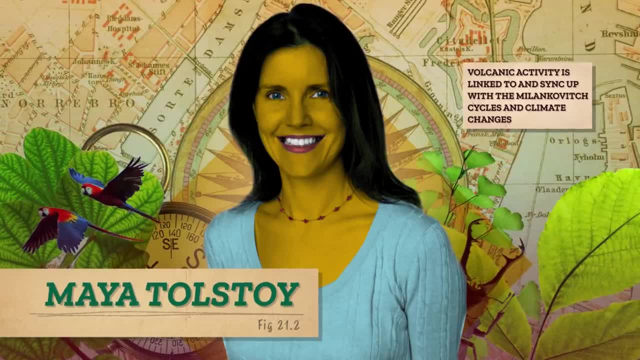 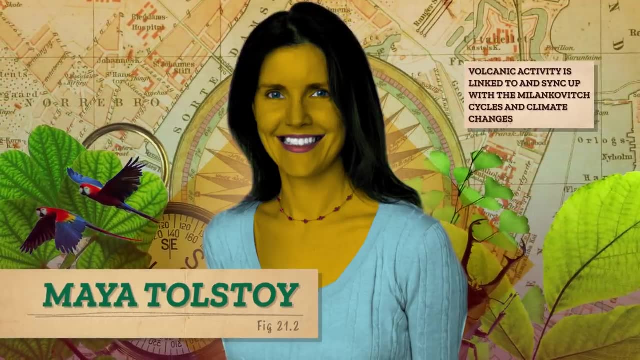 Earth Observatory think that whether land volcanoes will be more active than underwater volcanoes or the other way around, and when they will erupt are linked to and sync up with the Milankovitch cycles and climate change. During a glacial period, terrestrial volcanoes don't erupt as much because the weight of 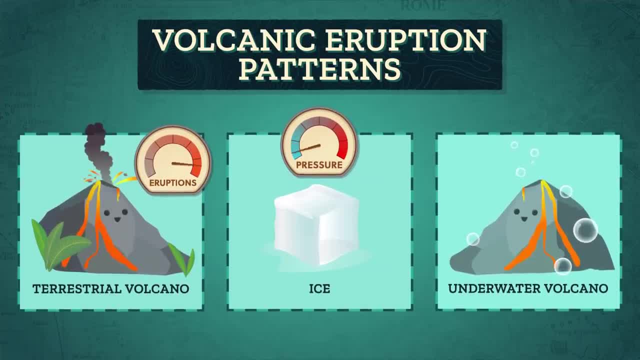 the ice on land puts pressure on the volcanoes. When the ice melts, the pressure lowers and we get more eruptions as all the material locked inside tries to escape. But underwater volcanoes are the opposite. As water turns to ice and the sea levels drop during a glacial period, the pressure on them 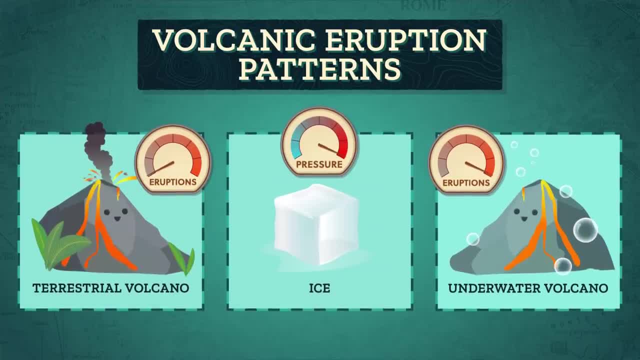 eases Rate is really important here, and modeling suggests that the faster the sea levels drop, the more eruptions we may get from underwater volcanoes. But correlation doesn't mean correlation And the timing here is complicated. Like underwater eruptions seem to start increasing when the sea level hits its lowest point. 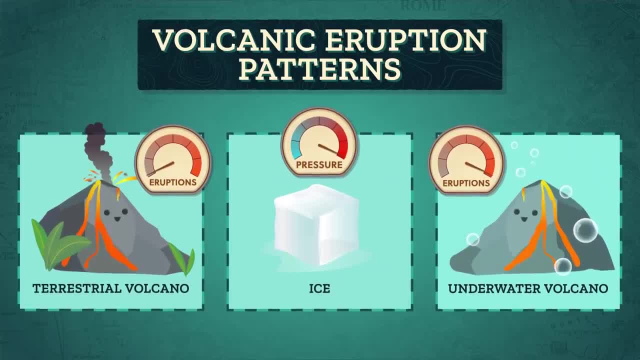 so, after the sea level has been going down for about 80,000 years. Scientists are still trying to figure out how volcanoes and climate change are related and what the timing means, and there's a lot of modeling going on. What's more astonishing is that underwater volcanoes not only respond to the changes. 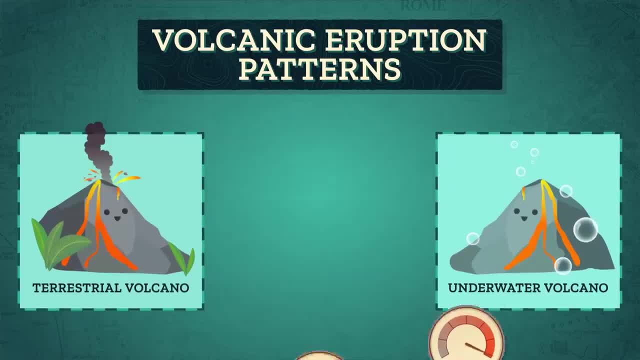 in sea levels associated with glacials and interglacials, but also to short-term sea level changes from ocean tides every few weeks. Changes in the shape of Earth's orbit could also be an important timing factor. When the orbit is more elliptical, the Sun's gravitational pull changes more rapidly and 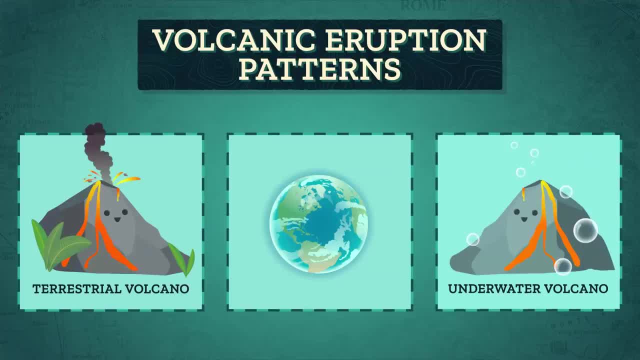 the Earth is squeezed and unsqueezed like an accordion, And we think this causes more undersea eruptions for a couple of reasons. Either the squeezing and unsqueezing generates more magma, kind of like how a paperclip gets hot when you bend and unbend it over and over, or the squeezing opens, cracks up more and 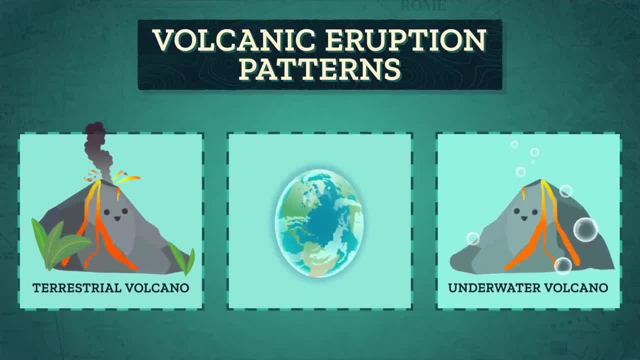 magma can move up more effectively And as the orbit becomes more circular as part of the 100,000 year cycle, this effect is dampened. There may be fewer undersea eruptions And, last but not least, all modern, well-documented mid-ocean ridge eruptions have occurred during.